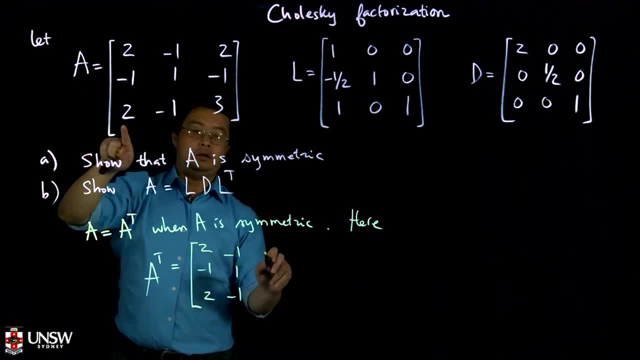 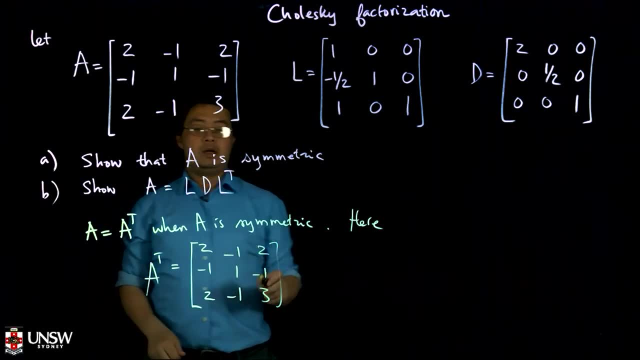 1, and 1, minus 1,, then 2, minus 1, and 3.. So you transpose all the rows into the columns And now you check. So now it's the same at the matrix A. Okay, so the same at matrix. 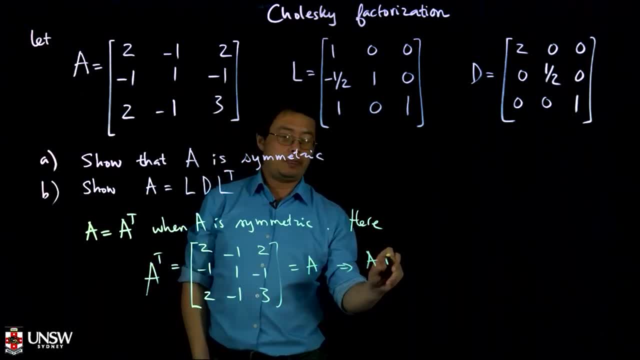 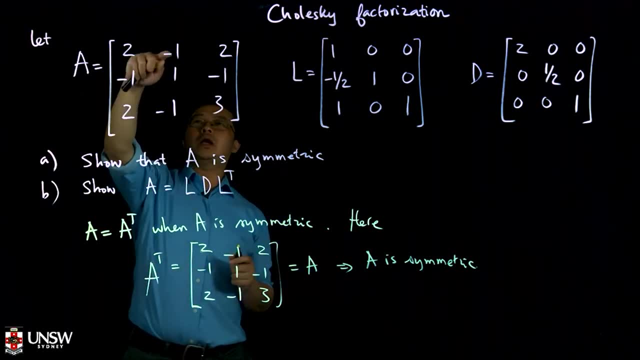 A, So A is symmetric. Another way to see it is: you know, you just check the entries opposite the diagonals. So minus 1 here and the same, minus 1 here. 2 and 2 here minus 1, minus 1 here, So they're the same. 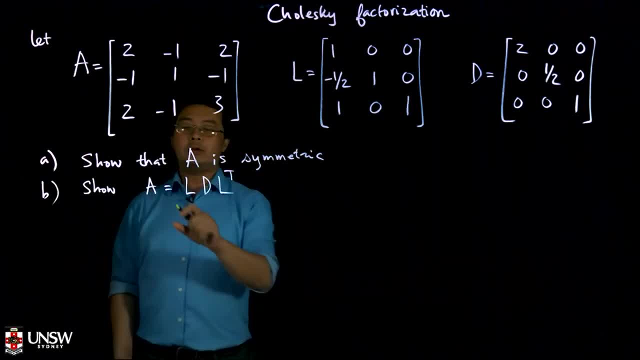 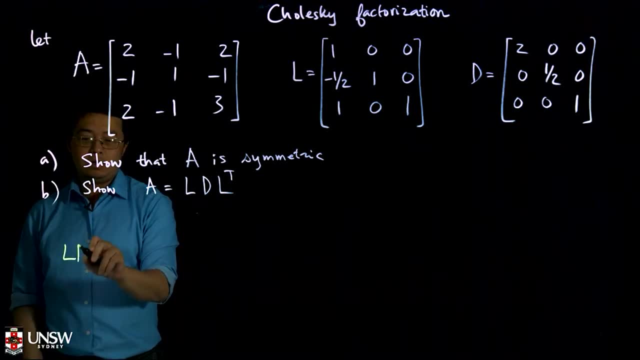 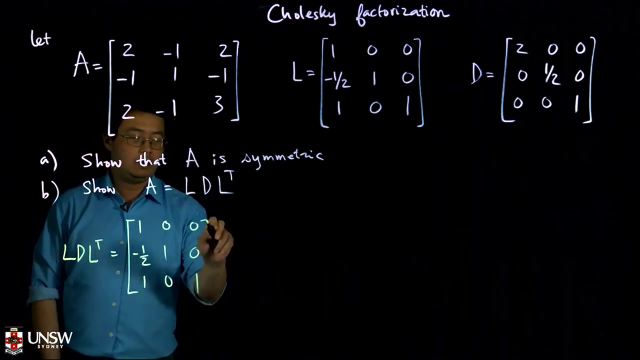 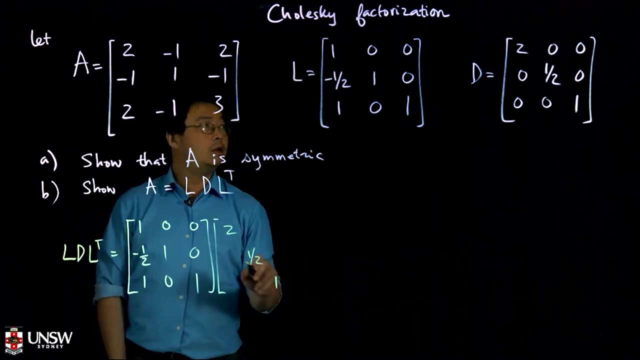 So that's symmetric. Okay, so now suppose I want to show that A is a product of L D, L transpose. So I just take L D, L transpose, L transpose to be so 1, minus 1, half 1, 0, 1, 0, 0, 0, 1.. And I multiply with the matrix D, So 2, 1, half 1, 0 here, 0 here, 0 here 0, 0, 0.. 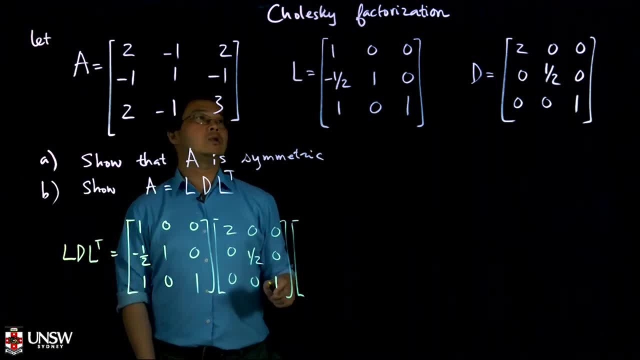 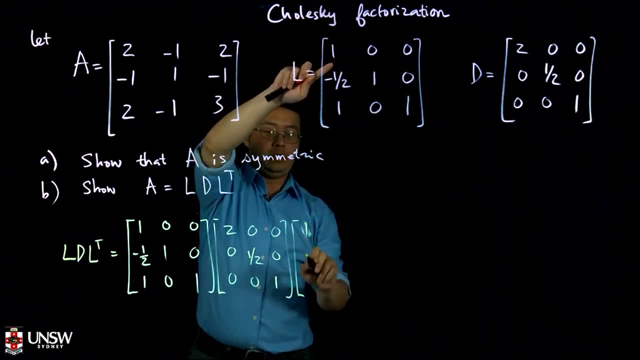 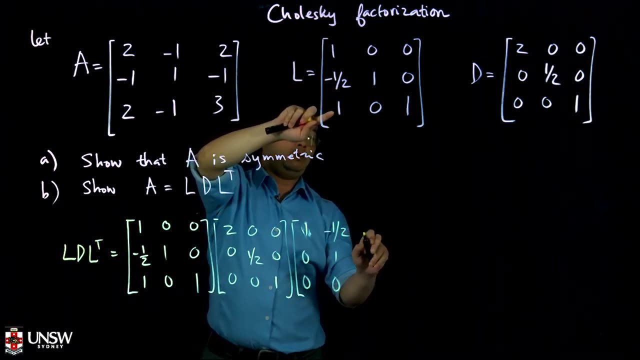 And then L transpose, So L transpose. I take the row become a column, So that will be 1, 0, 0, then minus 1, half 1, 0, then 1, 0, 1.. 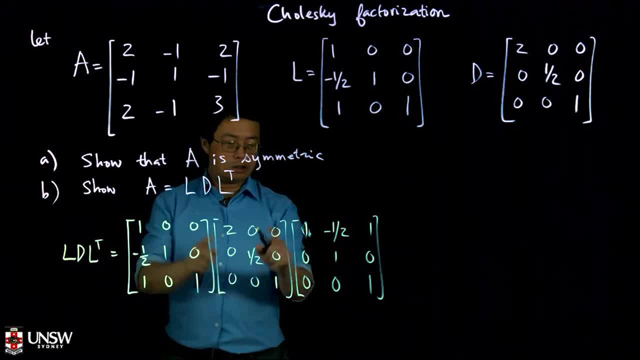 Okay, and then we multiply maybe this two matrix: first Okay, and then after that we multiply by this one. So here suppose I got 2 times 1 here and then 0, 0. So give me 2, and then 0 times 1.. 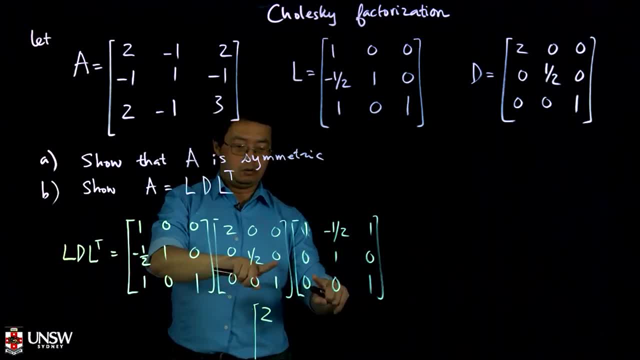 So 1, half times 0.. So 0 times 0. So give me 0.. The third one is: 0 here, 0 here, 0 here. So I have 0 here, Okay, and then I do the second row. So 0 times 1 is 0.. 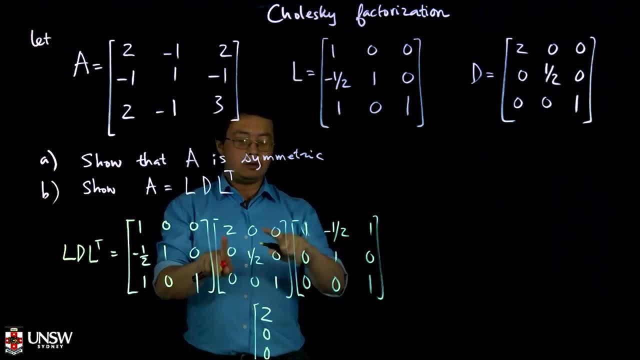 And then- Sorry, I have to do the second column. So second column is 2 times minus 1, half. It's minus 1.. Yeah, And then 0, 0.. So minus 1.. And the second column, second row, second column. So 0 here, then 1, half, then 0.. 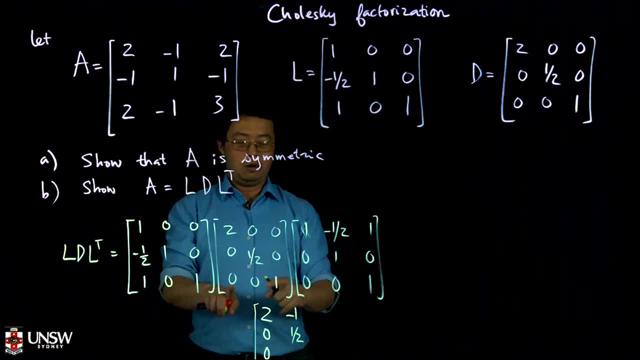 So 1, half here And the third row. so you got 0 here, 0 here, Then 0 here And now for the last columns. So now 2, 0, 0.. So we got 2.. 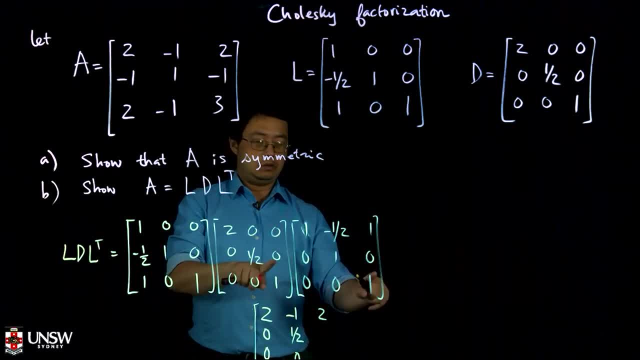 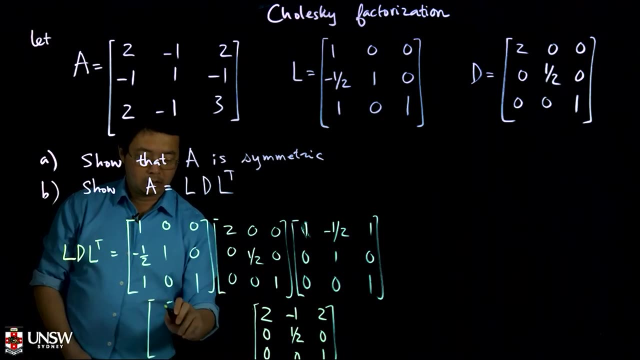 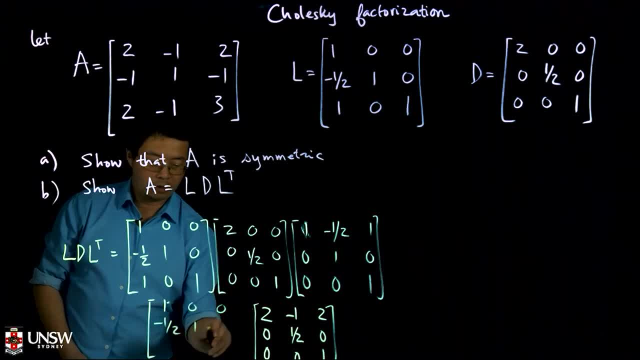 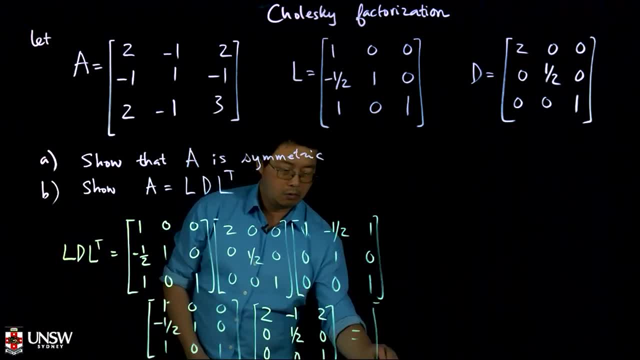 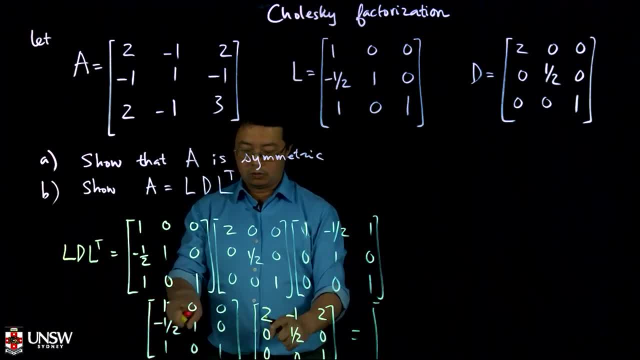 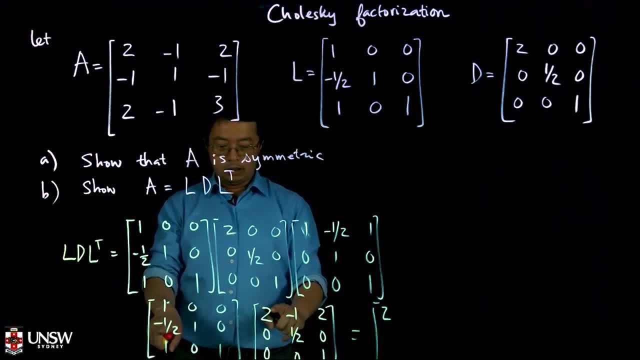 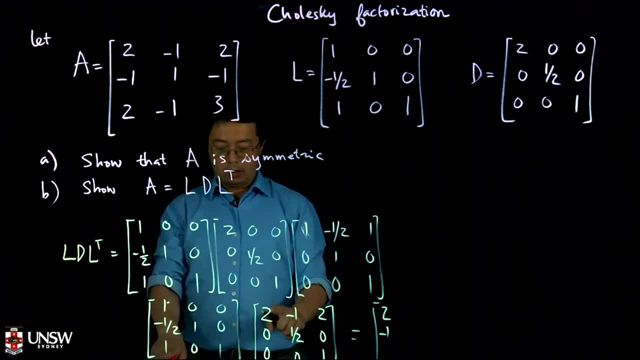 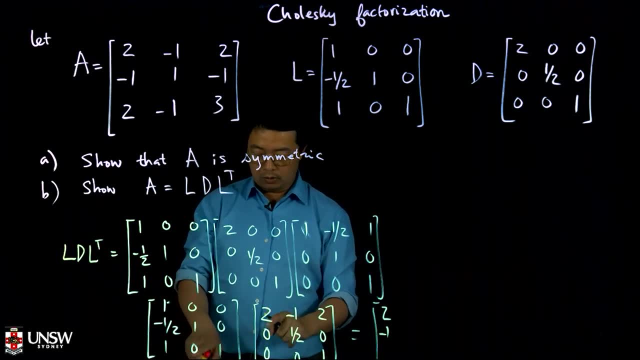 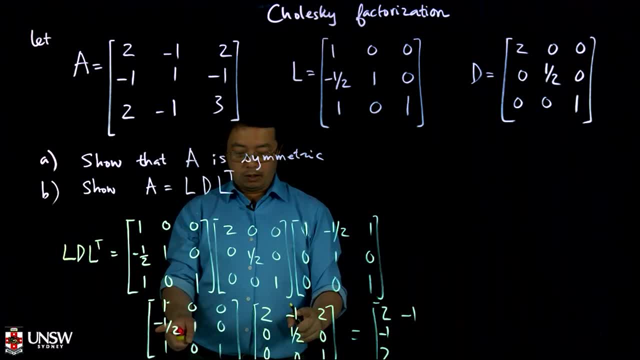 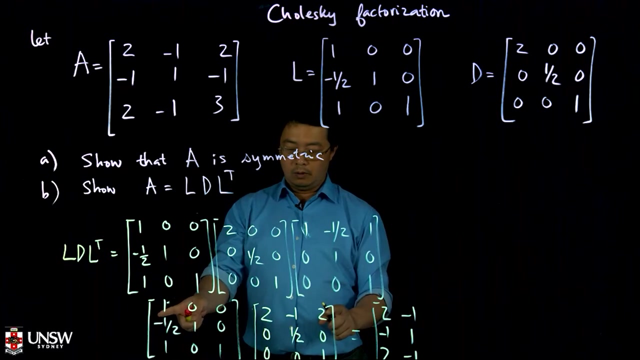 The second row, second column, so minus 1. half times minus 1 is plus 1.. So plus, sorry- plus one half and this one plus one half, so give me one. and the third row, second column, so minus one, zero, zero. so minus one here, and then the last one, so two, zero, zero, so two here. 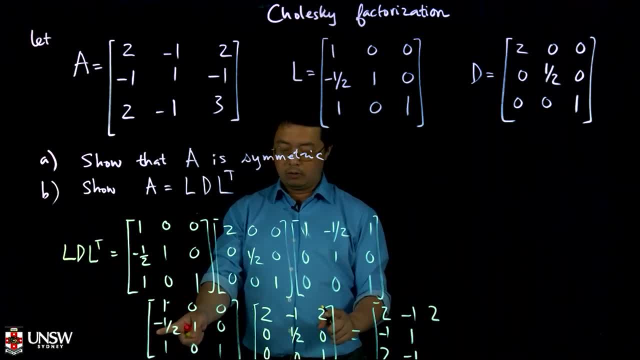 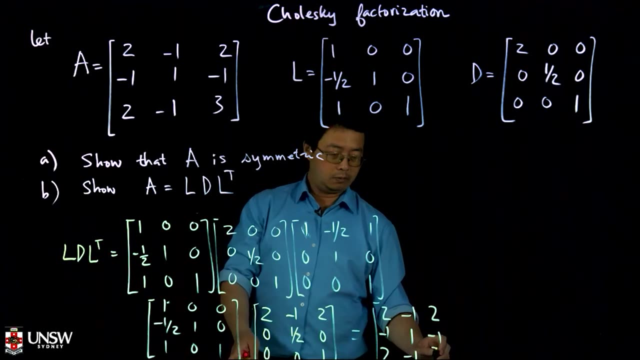 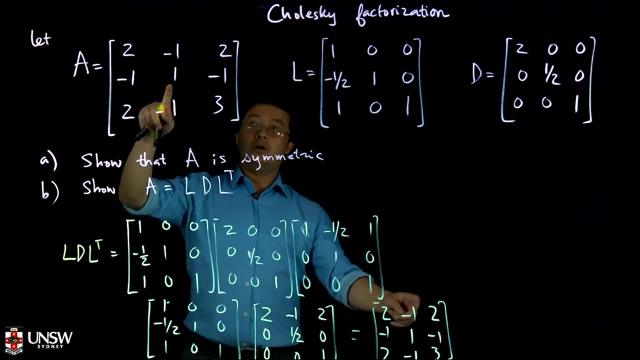 and the second row. so minus one. half time two is minus one, zero. zero, so minus one. and then the last one: one time two is two zero one. one, so three. so is it the same as original matrix? so two minus one. two minus one. one minus one. two minus one, three, so it's the. 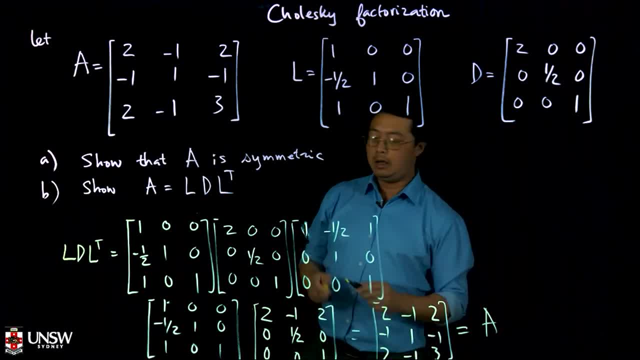 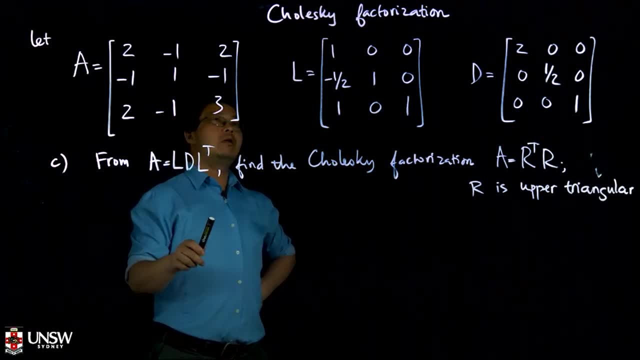 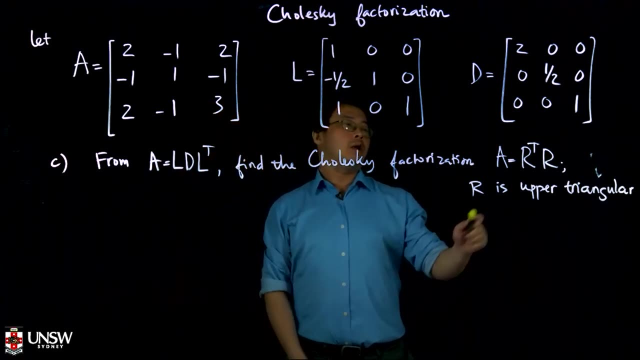 same as the matrix a, so we verify it by direct calculation. okay, so now we are going to find the Cholesky factor, the Cholesky factorization of the matrix a, given this identity. so remember, the Cholesky factorization is when you can draw a matrix as a product of a matrix. r transpose r when r is. 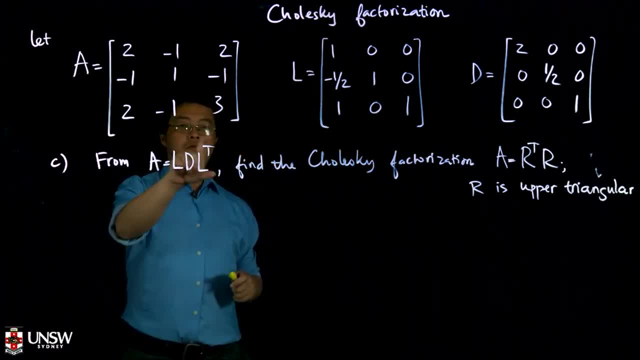 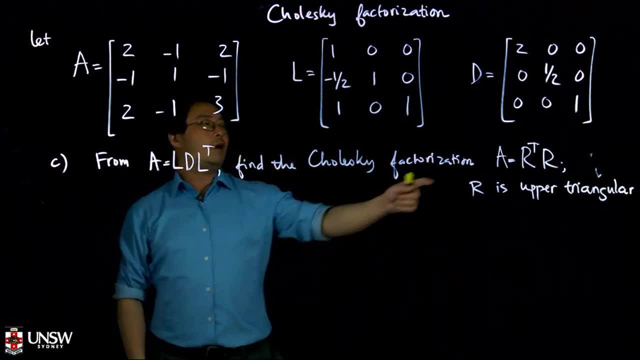 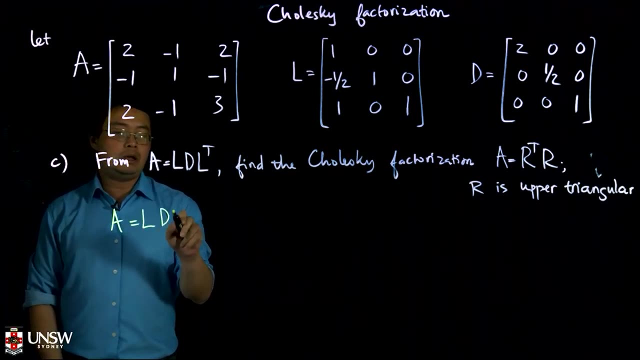 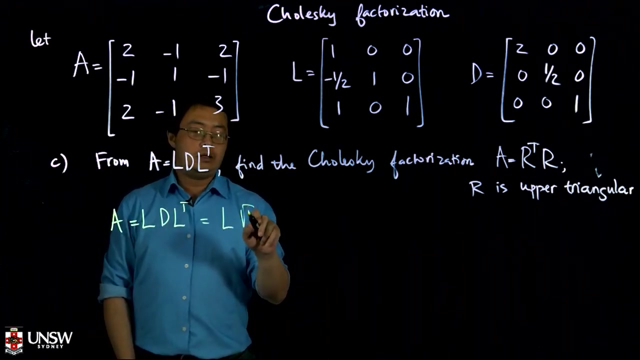 the upper triangular matrix. and now we make use of the previous equations- i mean a equal l, d, l transpose, in order to find out the Cholesky factorization. so now, suppose i write a, a, a equal l, d, l transpose. but now i want to split the matrix d into square root of d times square. 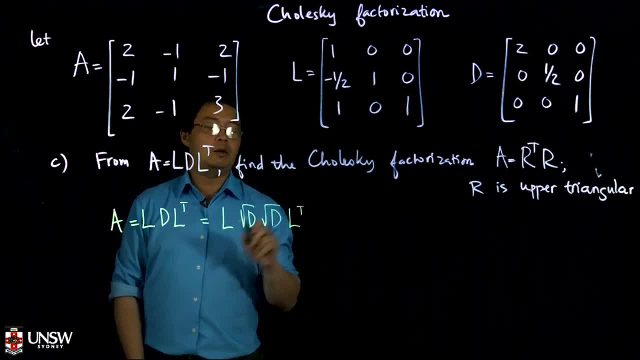 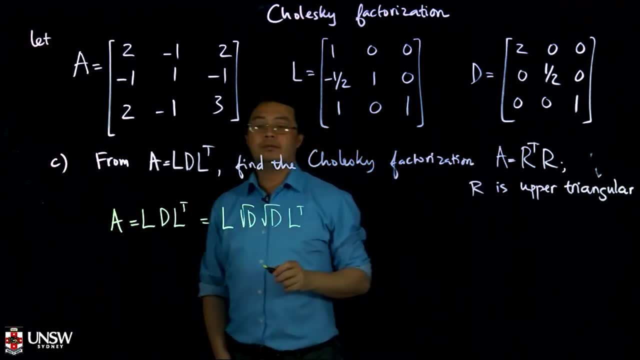 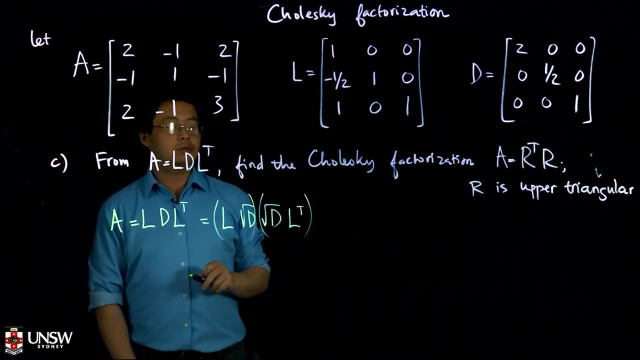 root of d times l transpose. okay, and remember the matrix d is diagonal, so the square root of d is just the square root of all the entries, okay. and then now i combine this: uh, two products, you know, just the square root of all the entries, okay. and then now i combine this: uh, two products, you know. 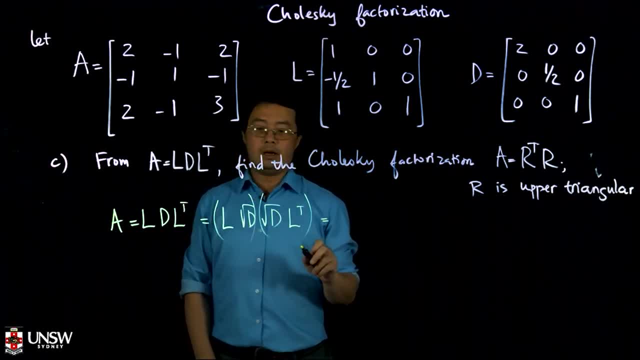 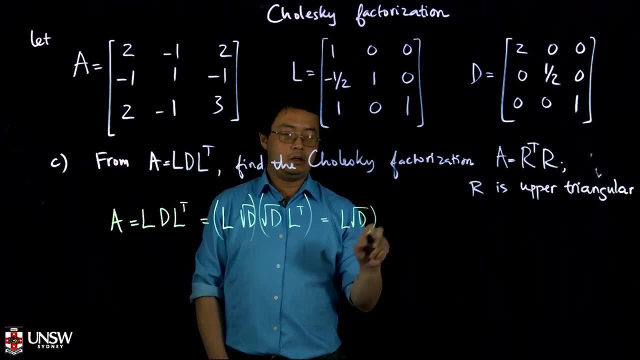 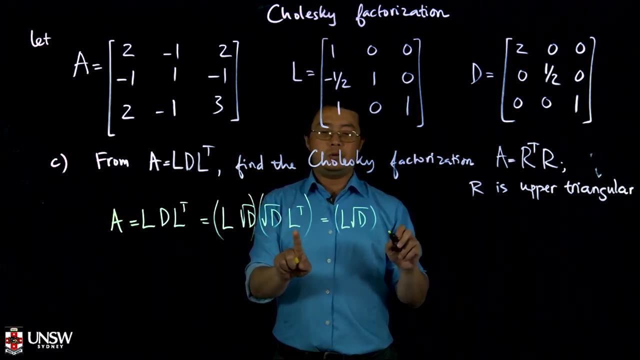 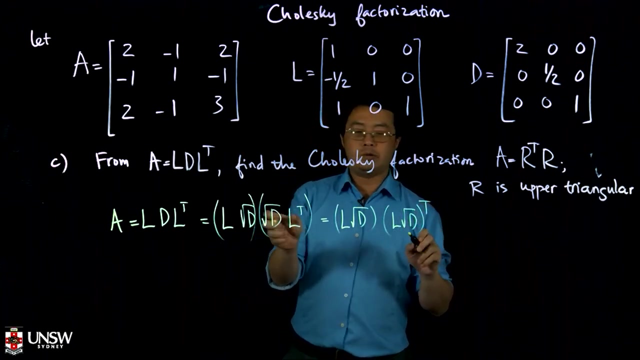 so then i can draw this one is the: uh, l transpose. i mean l square root d time. so remember the matrix: square root d, l transpose. it could be written as l and square root d everything, transpose. because when you transpose then you got like square root d, transpose what is the same square root d. 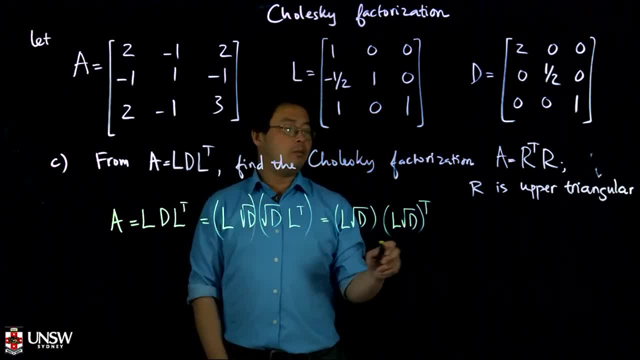 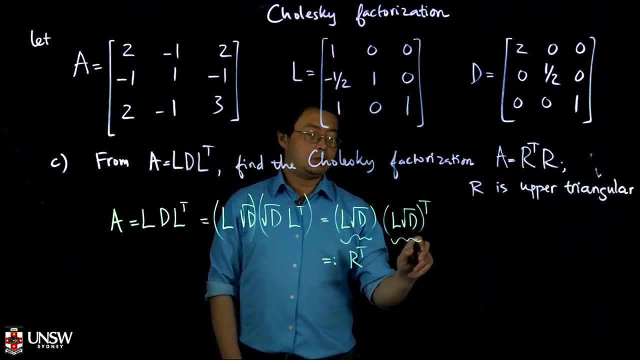 because when you transpose, then you got like square root d and l transpose, and now i will label and l transpose, and now i will label this matrix to be r- transpose. okay, i label this and this matrix, this matrix to be r- transpose. okay, i label this and this matrix will be the matrix r. 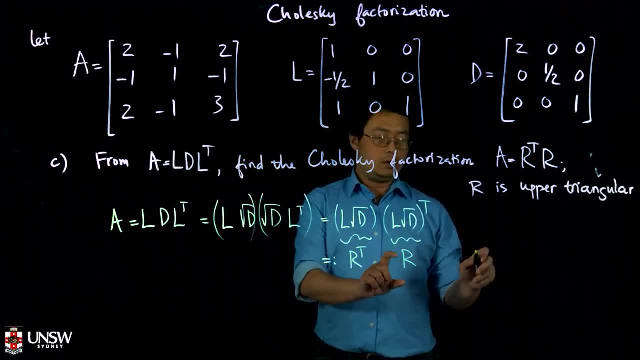 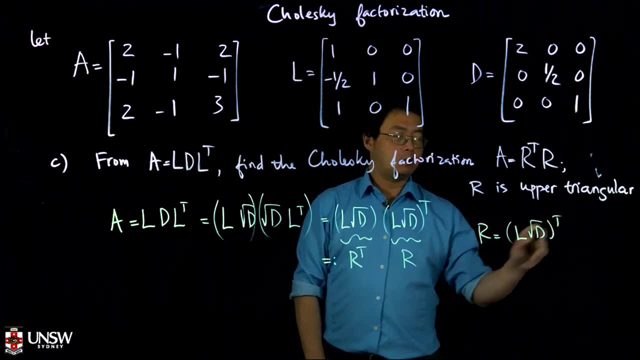 will be the matrix r. okay, and so you can see that. if i read: if i, if i set r equal, okay, and so you can see that. if i read: if i, if i set r equal l square root d transpose, then r transpose l square root d transpose, then r transpose, it just equal l square root d. 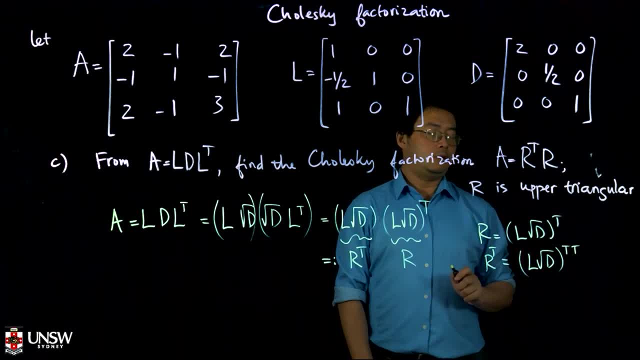 it just equal l square root d transpose, then r transpose it just equal l square root d transpose, then r transpose it just equal l square root d. it just equal l square root d transpose, then r transpose it just equal l square root d transpose, transpose, transpose, transpose. yeah, and what is just the same as l. 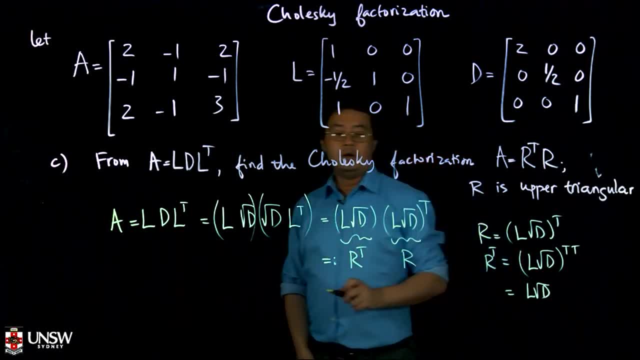 yeah, and what is just the same as l. yeah, and what is just the same as l square root d. square root d. square root d. what is here l square root d, so now i have. what is here l square root d, so now i have. what is here l square root d, so now i have r equal. 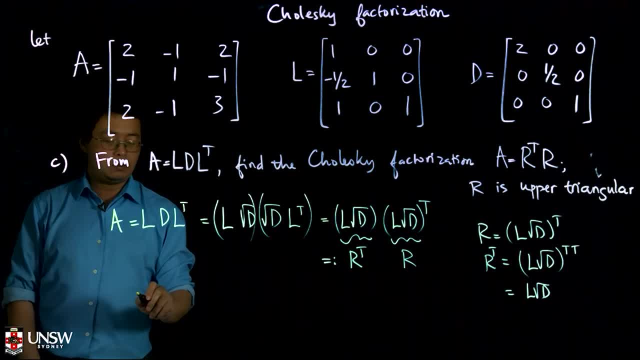 r equal r equal l square root d. so now i just compute the l square root d. so now i just compute the l square root d. so now i just compute the product l times square root d. so l product l times square root d. so l product l times square root d so l square root d. 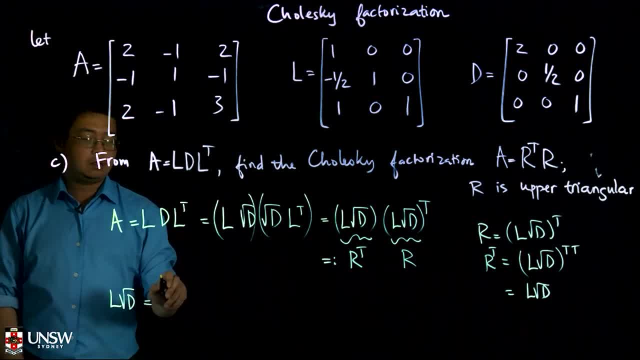 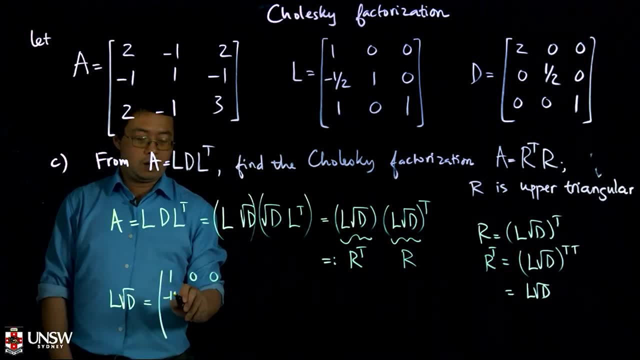 square root d, square root d will equal, will equal, will equal. so now this one is, so now this one is, so now this one is. the matrix l here, so one. the matrix l, here, so one. the matrix l here, so one: zero, zero, zero, zero, zero, zero. then minus one half. 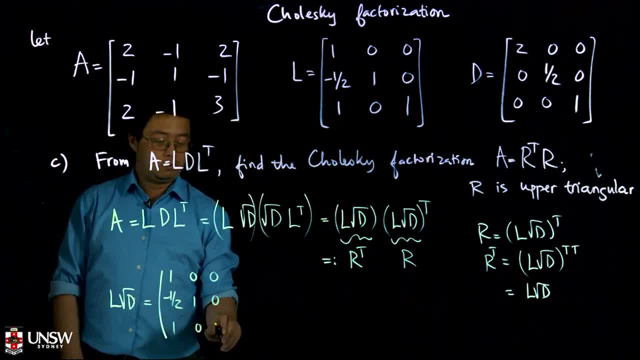 then minus one half, then minus one half: one zero one, zero one. zero one. one, zero one, one, zero one. and the matrix d square root d will be, and the matrix d square root d will be, and the matrix d square root d will be square root two. 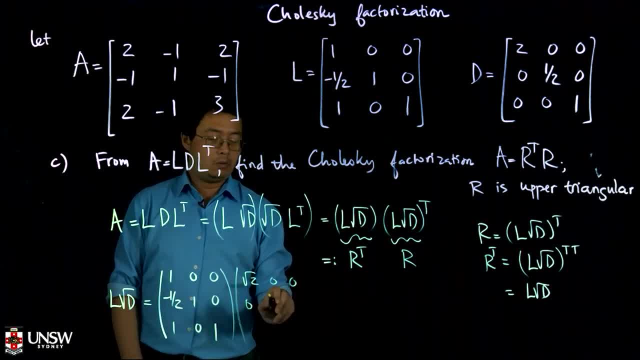 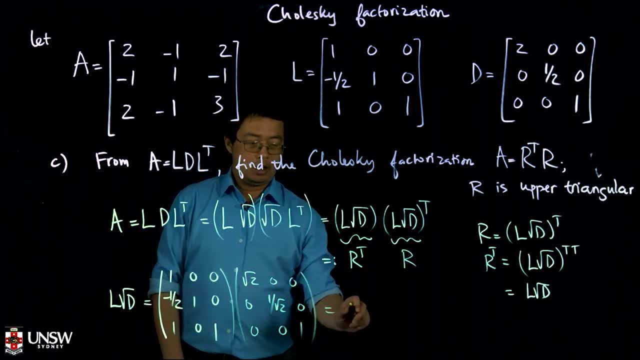 square root two, square root two. zero, zero, zero, zero, zero, zero, and then zero one over square root two, and then zero one over square root two, and then zero one over square root two. zero, zero, zero, zero, one, zero, zero one, zero, zero one. and now i just multiply it out. 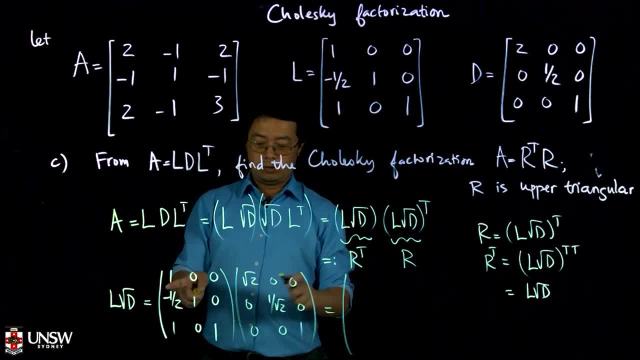 and now i just multiply it out, and now i just multiply it out, and and now i just multiply it out, then i have, then i have, then i have. so one times square root two is square. so one times square root two is square. so one times square root two is square root two. 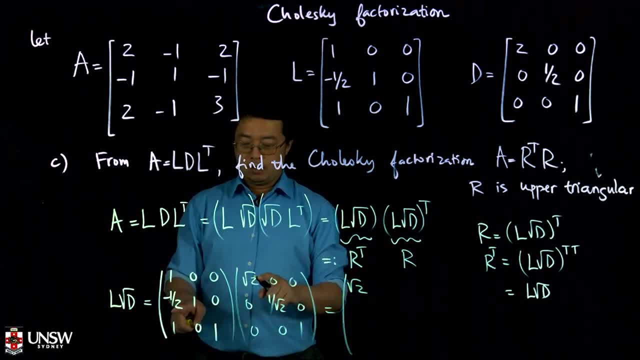 root two root two and zero zero, so and zero zero, so and zero zero. so then then then minus, minus, minus one half times square root two. one half times square root two. one half times square root two is minus one over root two is minus one over root two. 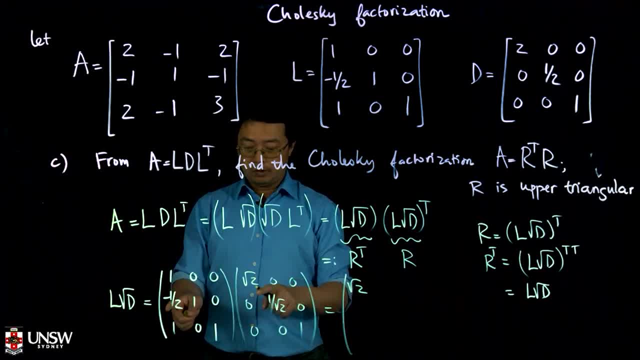 is minus one over root two. okay, okay, okay, and and and zero, zero, so zero, zero, so zero, zero, so minus, minus, minus one over root two, one over root two, one over root two, and then the last row is one time root and then the last row is one time root. 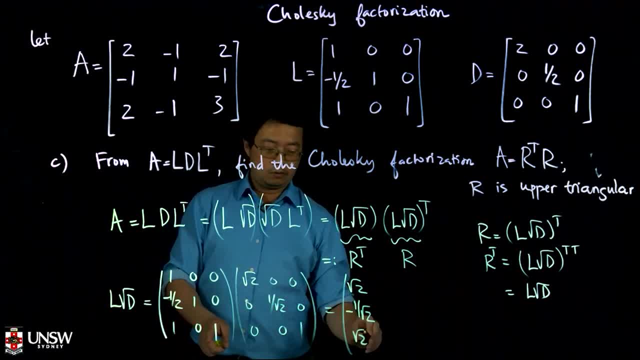 and then the last row is: one time root two and and zero, zero. so you have root two here, zero, zero. so you have root two here, zero zero. so you have root two here, and then after that i have, and then after that i have, and then after that i have. the second column is: i just take the. 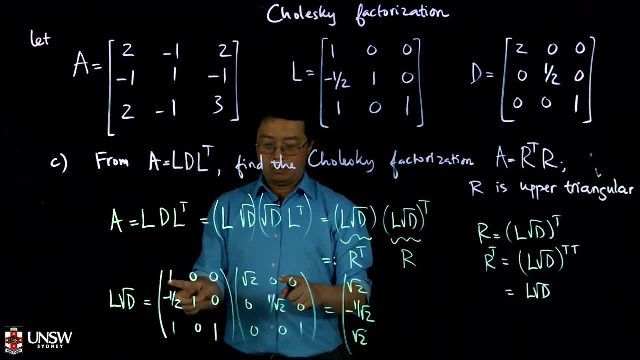 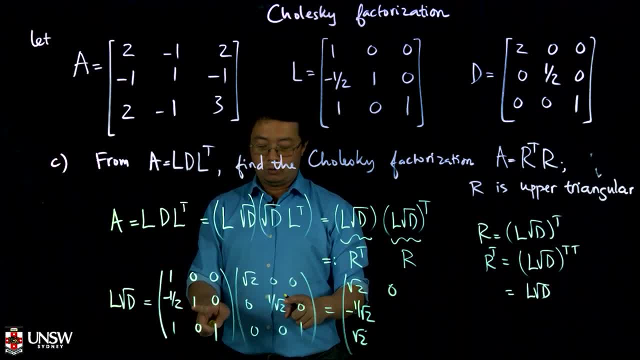 and now second. and now second row, second column. so zero here row, second column, so zero. here row, second column. so zero here and one over root two and zero. so one and one over root two and zero. so one and one over root two and zero. so one over root two. 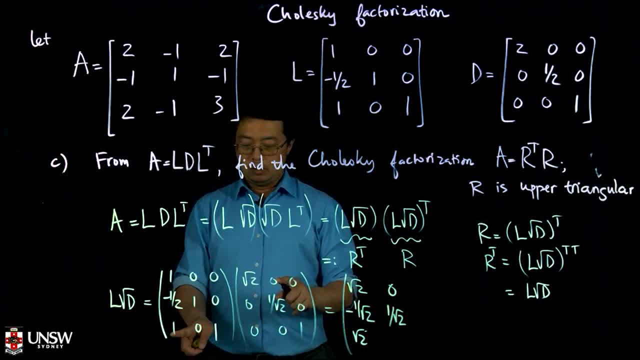 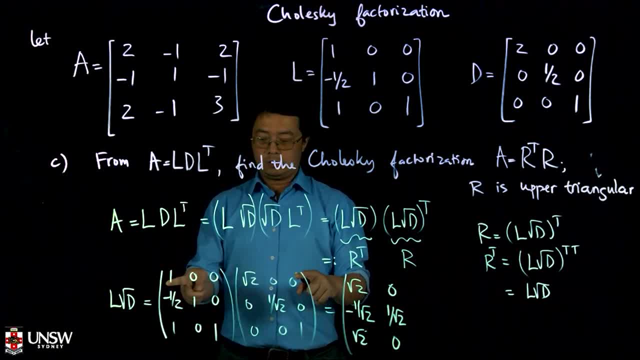 and for the last column i just take the. and for the last column i just take the first row. first row, first row, and then last column here, so zero here. and then last column here, so zero here. and then last column here, so zero here, zero here, zero here. 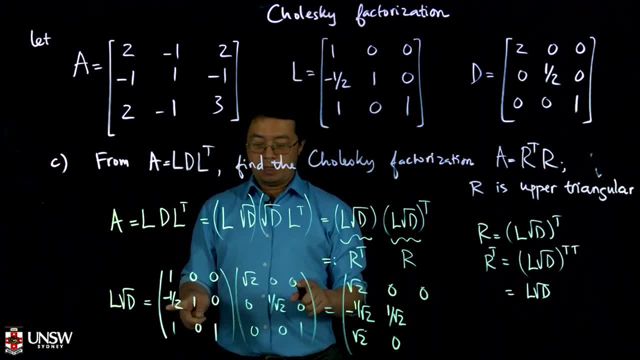 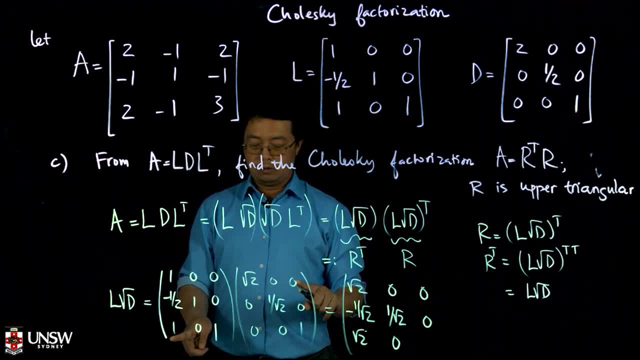 and now the last. and now the last column, last column, last column, last row: row, row. so one times zero, so one times zero, so one times zero, zero, and then one zero, and then one zero and then one. so you can see that this is a matrix r. 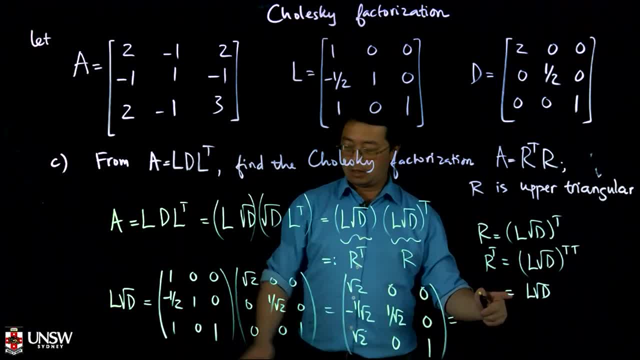 so you can see that this is a matrix r. so you can see that this is a matrix r. transpose, transpose, transpose. yeah, because r transpose is l. yeah, because r transpose is l. yeah, because r transpose is l square root d, square root d, square root d. and from here then you can get out the. 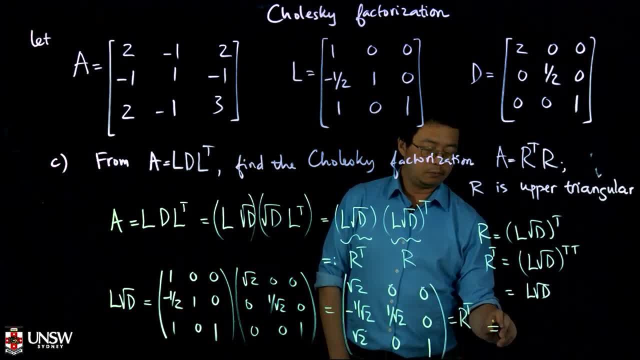 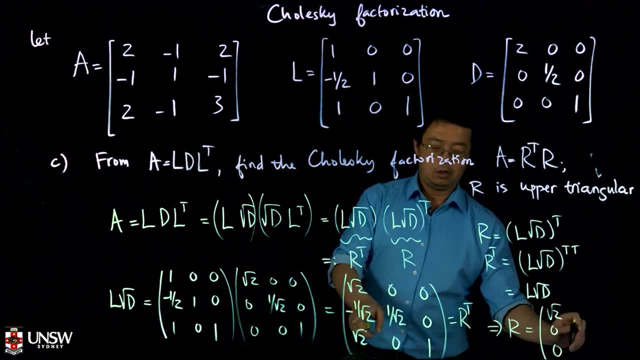 and from here then you can get out the and from here then you can get out the matrix r, matrix r, matrix r, so the matrix r will be. you just take this one, you transpose it. you just take this one, you transpose it. you just take this one, you transpose it, so you got square root, two zero zero. 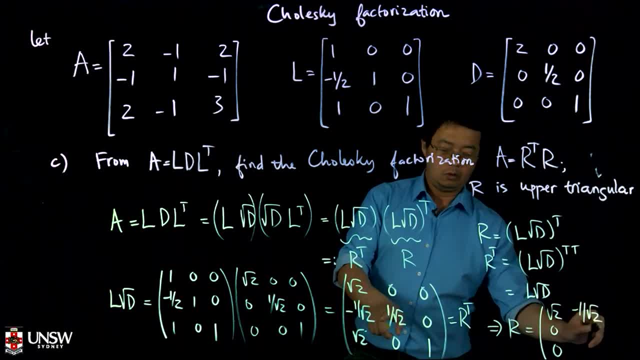 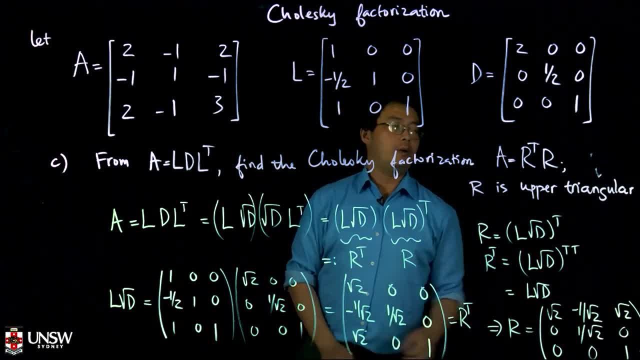 and then the last one will root 2 0 1, and then the last one will root 2 0 1. so you can see that the matrix r is. so you can see that the matrix r is. so you can see that the matrix r is upper triangular matrix. 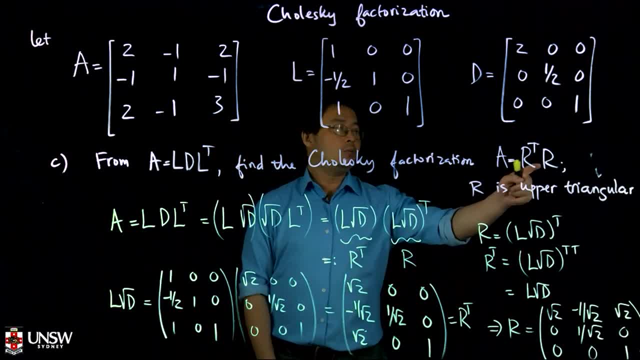 upper triangular matrix, upper triangular matrix. and you can verify that if you take r. and you can verify that if you take r. and you can verify that if you take r, transpose multiply by r, transpose multiply by r, transpose multiply by r and you recover the matrix a again. 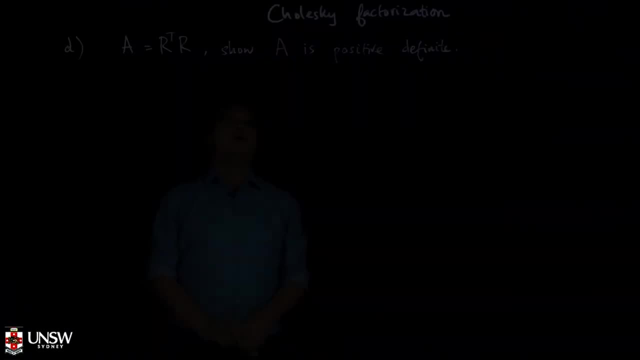 and you recover the matrix a again, and you recover the matrix a again, and this is called the cholesky, and this is called the cholesky, and this is called the cholesky. factorization, factorization, factorization. okay, so now we will show that. 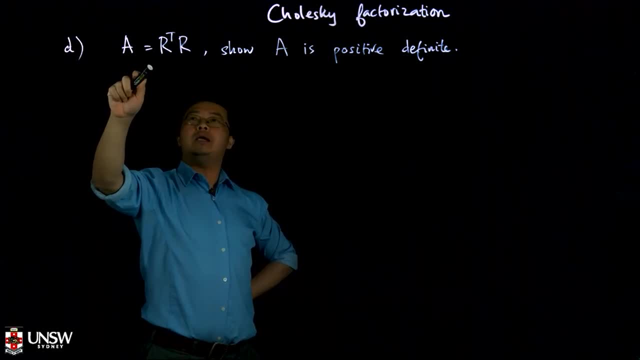 okay, so now we will show that. okay, so now we will show that if you have a cholesky factorization, if you have a cholesky factorization, if you have a cholesky factorization, this means that when you can write a as, this means that when you can write a as: 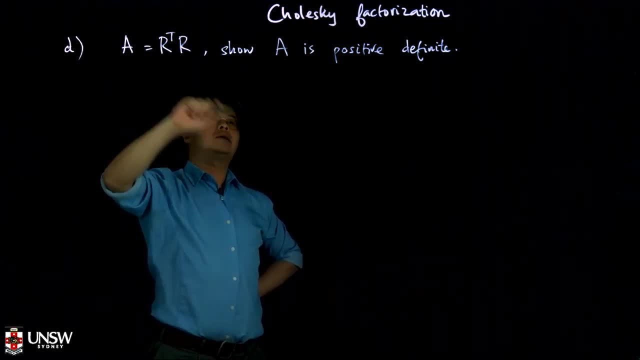 this means that when you can write a as a product, a product, a product of r. transpose r. r is upper triangular of r. transpose r. r is upper triangular of r. transpose r. r is upper triangular matrix, matrix matrix, and r is non-singular and r is non-singular. 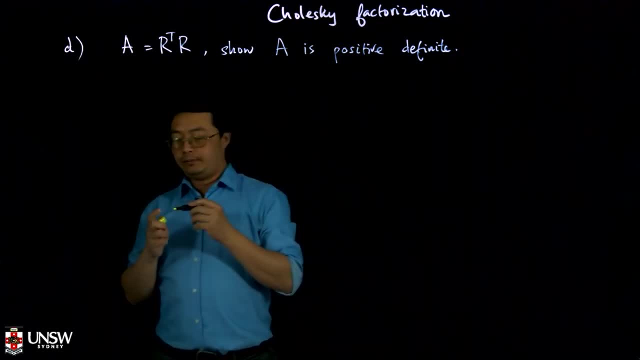 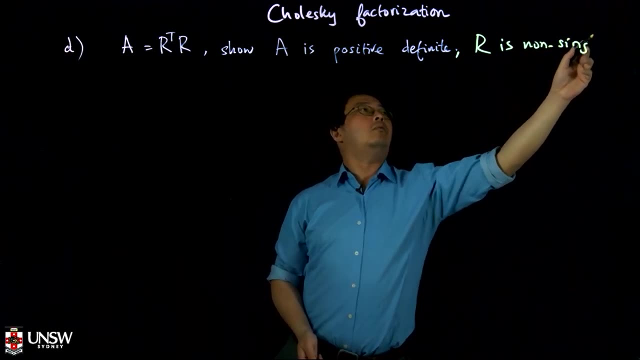 and r is non-singular. show that a is positive definite. show that a is positive definite. show that a is positive definite. so so r is non-singular, okay. so now, in order to show that a is okay. so now, in order to show that a is: 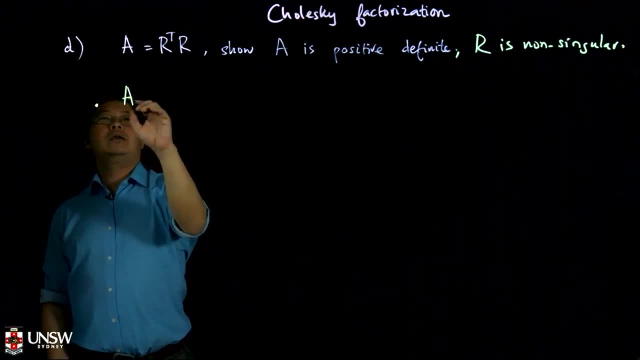 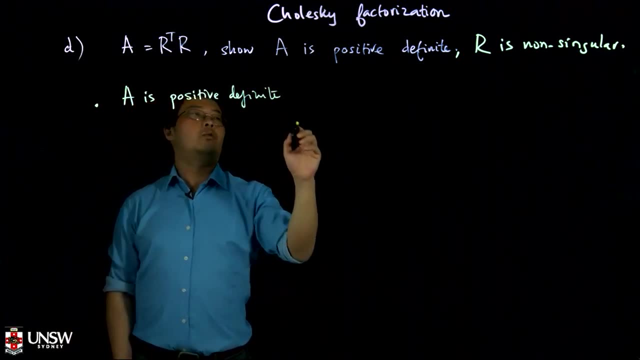 okay. so now, in order to show that a is positive definite, so now positive definite. so now positive definite. so now a matrix a, a matrix a. a matrix a is positive definite. my definition is when. my definition is when my definition is when you take x, transpose ax. 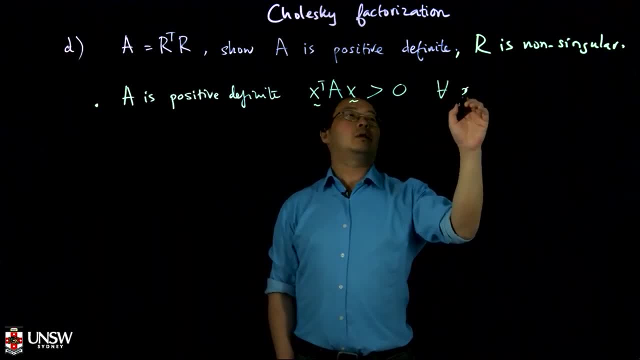 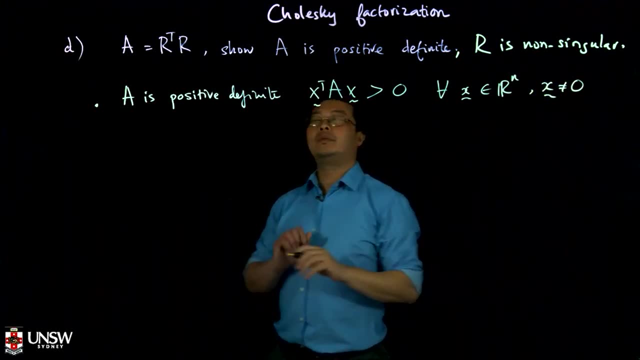 you take x transpose ax. you take x transpose ax, and this one is positive for all. and this one is positive for all and this one is positive for all. vector x, vector x. vector x. in in in a, in a rn, rn, rn, and, and, and the vector is non-zero. okay. 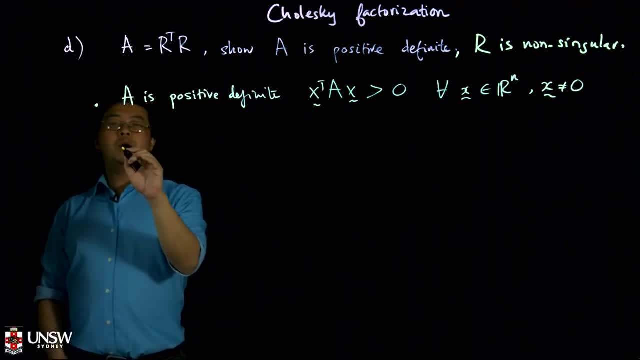 the vector is non-zero, okay, the vector is non-zero, okay. so we have to show that. satisfy this. so we have to show that. satisfy this. so we have to show that, satisfy this property. so now suppose i take x property. so now suppose i take x property. so now suppose i take x, transpose ax. 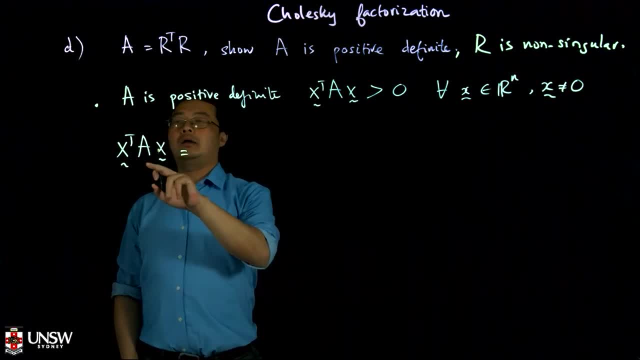 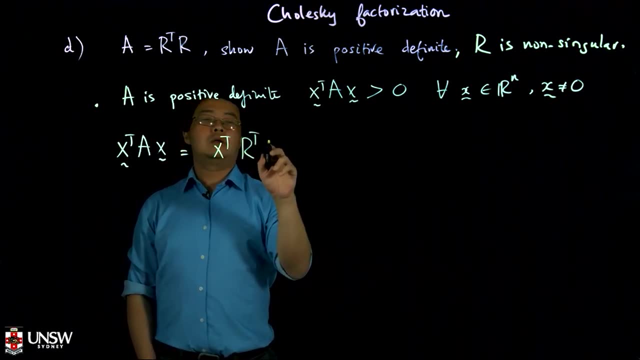 transpose ax, transpose ax. then, instead of writing x, transpose ax. then, instead of writing x, transpose ax, then instead of writing x, transpose ax, i replace a by r- transpose r. i replace a by r- transpose r. i replace a by r, transpose r, and i have x- transpose r, transpose. 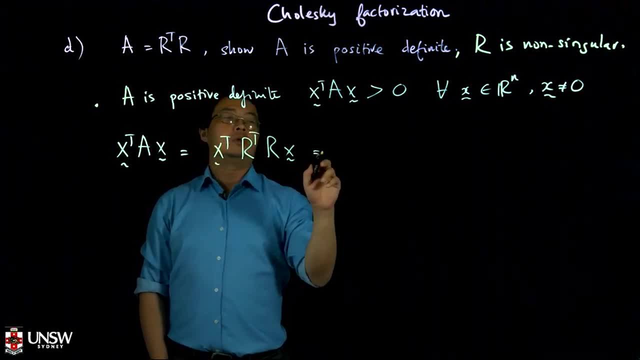 and i have x transpose, r transpose, and i have x transpose, r transpose, then r and x, then r and x, then r and x. okay, okay, okay, and so the first two terms i can rewrite, and so the first two terms i can rewrite. and so the first two terms i can rewrite as rx. 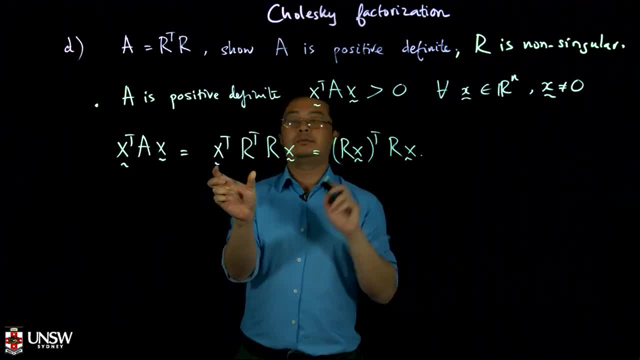 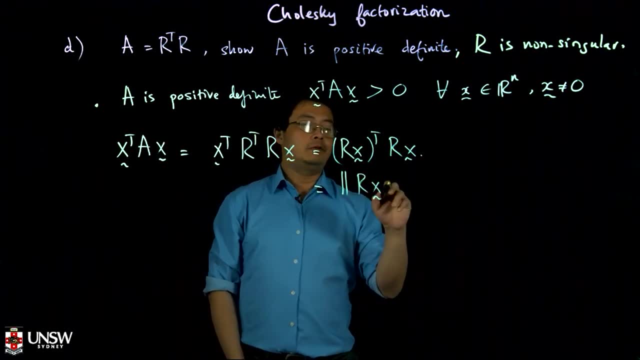 as rx, as rx, transpose, transpose, transpose, time rx, time rx, time rx. yeah, yeah, yeah. and now this one is nothing but the, and now this one is nothing but the, and now this one is nothing but the two norm, two norm. two norm of the vector: rx square. 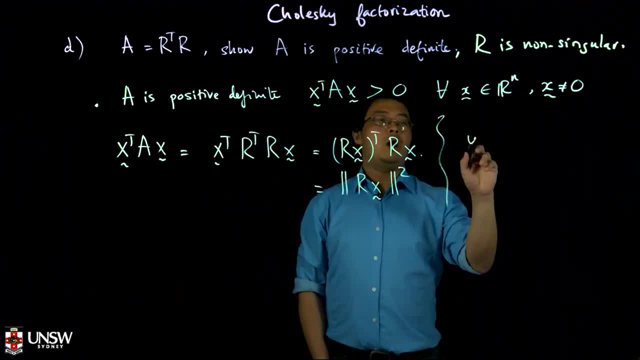 of the vector rx square of the vector rx square. okay, so remember, okay, so remember, okay, so remember: if you have y, transpose y. if you have y, transpose y. if you have y, transpose y, then this one is just y1, then this one is just y1. 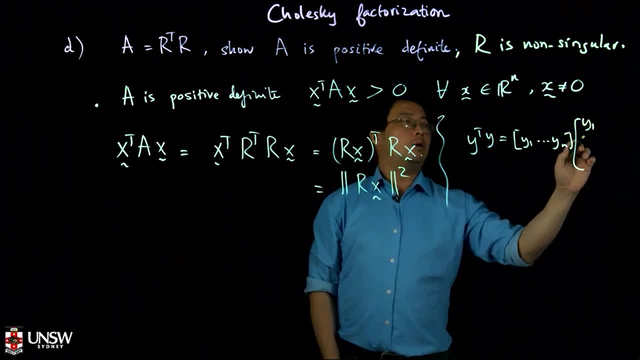 then this one is just y1 up to yn, up to yn, up to yn, and then multiply by the column, and then multiply by the column, and then multiply by the column. vectors y1 up to yn. vectors y1 up to yn. vectors y1 up to yn, and this one gives you y1 square. 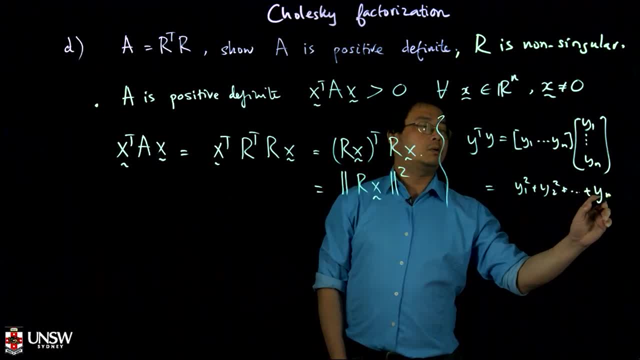 and this one gives you y1 square and this one gives you y1 square, y2 square up to y2 square up to y2 square up to yn square. and this one is just the two yn square and this one is just the two yn square and this one is just the two norm. 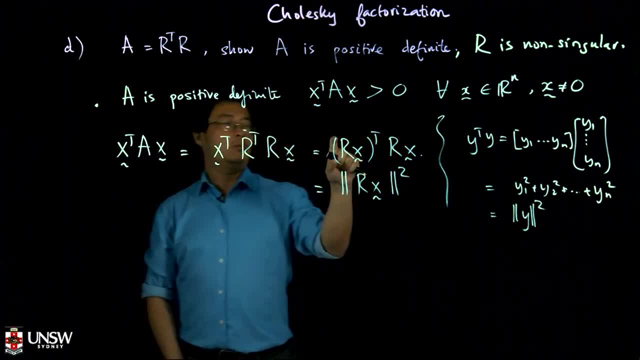 norm, norm, square of the vector y, so we use it square of the vector y, so we use it square of the vector y, so we use it right here. so the vector y right here, so the vector y right here. so the vector y just rx, okay. and you see, because this 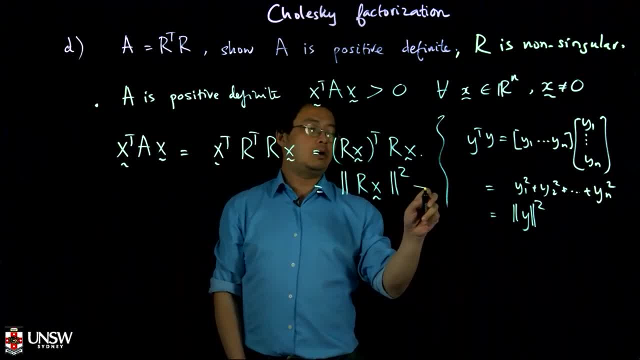 just rx, okay. and you see, because this just rx okay. and you see, because this one is square, one is square. one is square of some quantity, so it's greater, or of some quantity, so it's greater, or of some quantity, so it's greater, or equal zero. 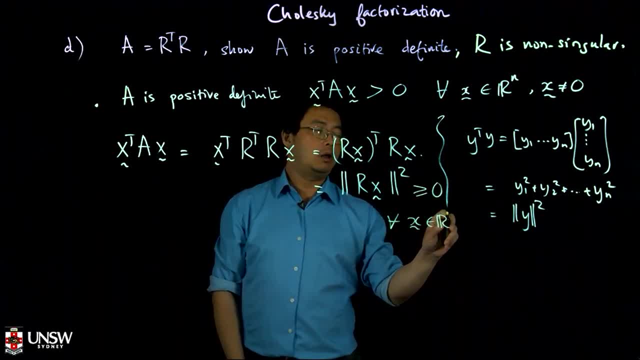 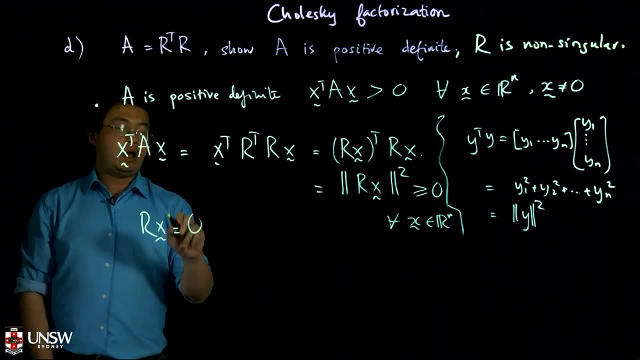 equal zero, equal zero for all vector x, for all vector x, for all vector x in rn, in rn, in rn. okay, okay, okay. so now, what happens if rx equals zero? so now, what happens if rx equals zero? so now, what happens if rx equals zero? so if rx equals zero because r is a. 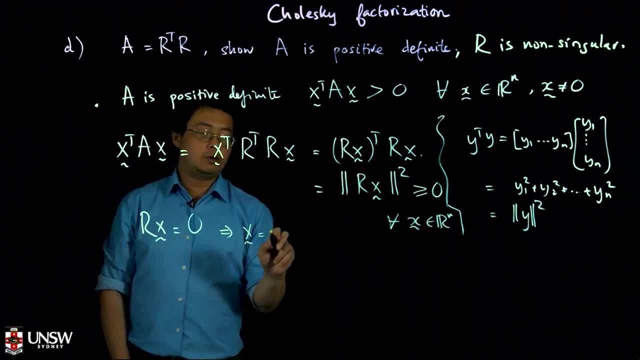 so if rx equals zero because r is a, so if rx equals zero because r is a non-singular matrix, non-singular matrix, non-singular matrix, so x has to be equal zero. so x has to be equal zero. so x has to be equal zero. so because 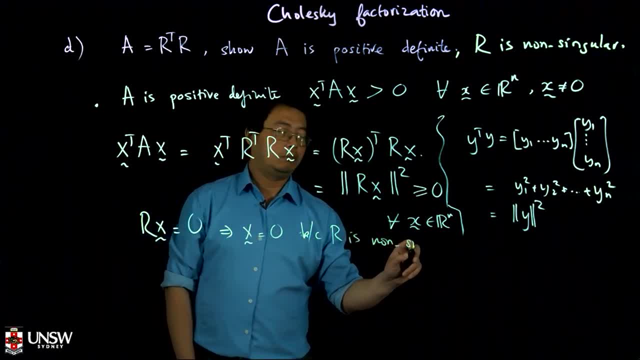 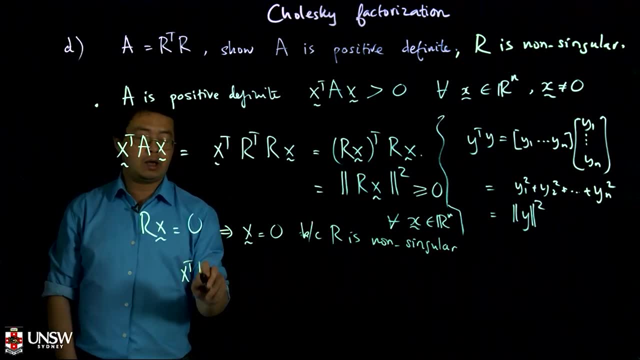 so, because, so, because r is non-singular, so, therefore, so, therefore, so, therefore, you, you, you know, you have shown that x transpose, know you have shown that x transpose, know you have shown that x transpose ax, ax. ax is always greater equal zero for all, is always greater, equal zero for all.